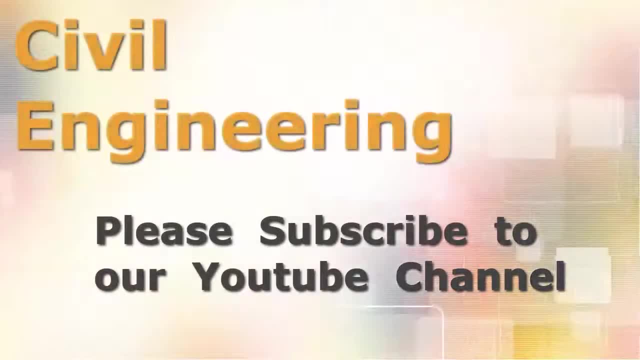 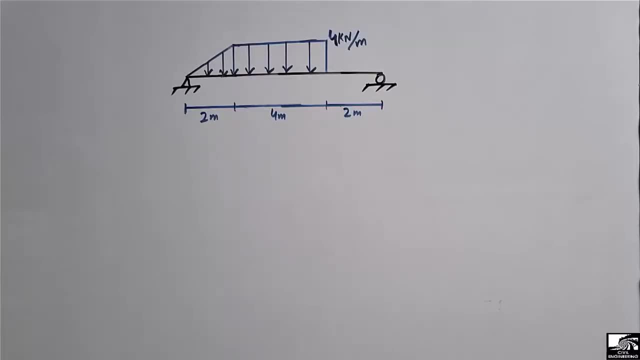 Hello guys, welcome back to the Civil Engineering YouTube channel. Please subscribe our channel for delicious civil engineering videos. In today's lecture we are going to find out the support reaction for this simply supported beam. This is a simply supported beam with a total length of 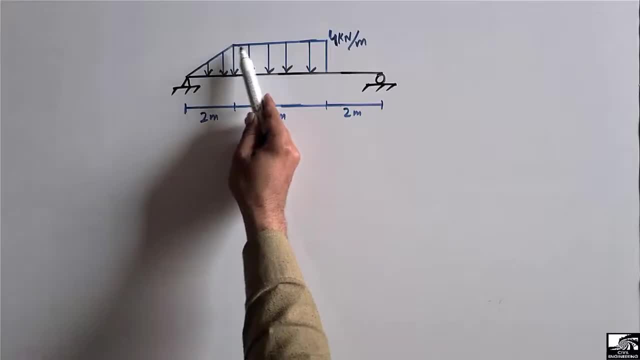 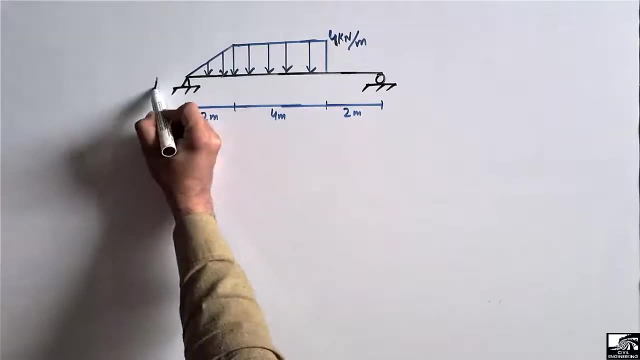 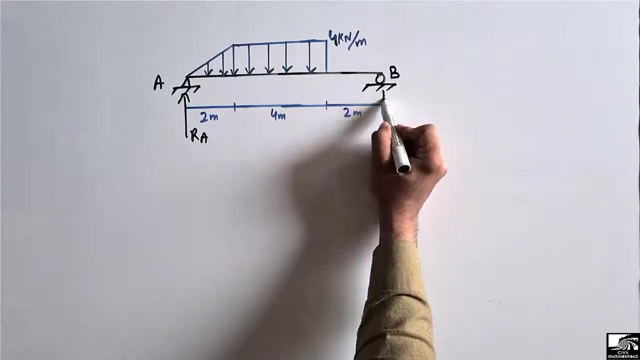 8 meter and it carries a triangular load and a rectangular load, So there is quite different loading acting on this beam. So we let's consider this is support A and this is support B and we are going to find out their support reaction- R A and R B. To start with the support reactions, 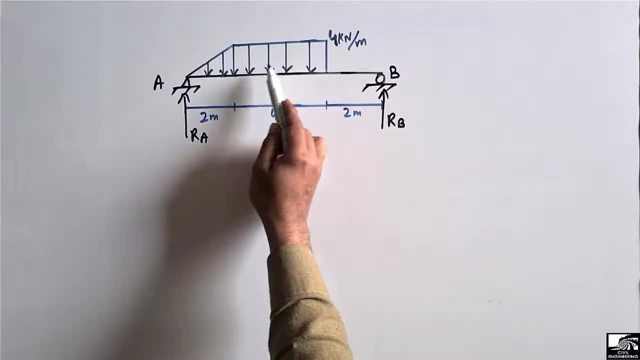 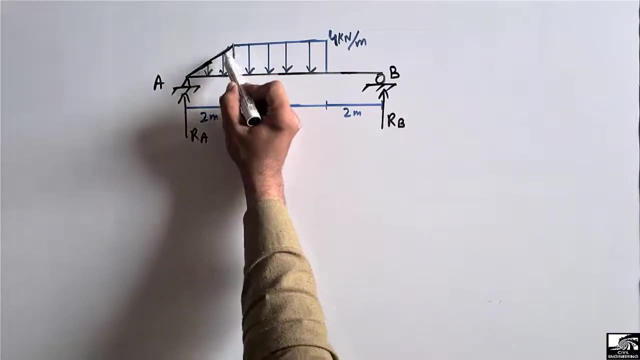 first we have to calculate their concentrated load. This is a uniformly varying load of triangular load. This is a triangular load, and then we have the rectangular load. So here we have the rectangular load, and then we have the rectangular load. So here we have. 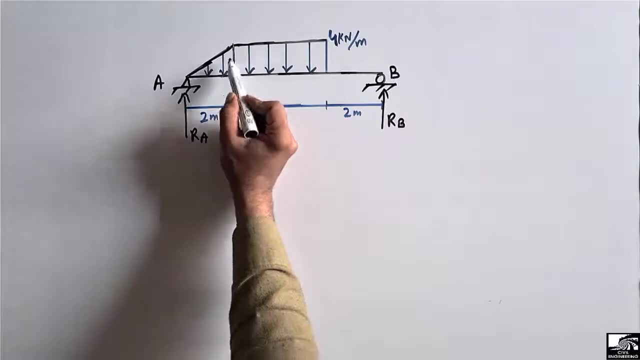 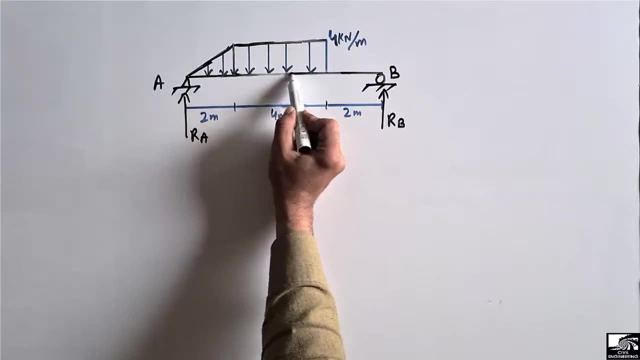 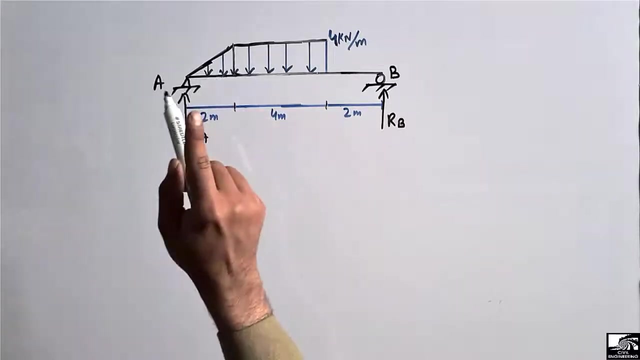 the triangular load is up to the distance of 2 meter, and then we have the rectangular load from 2 meter up to the distance of 4 meter. So there is a rectangular load. So we have one triangular load and one rectangular load. So first we have to find out the load, the 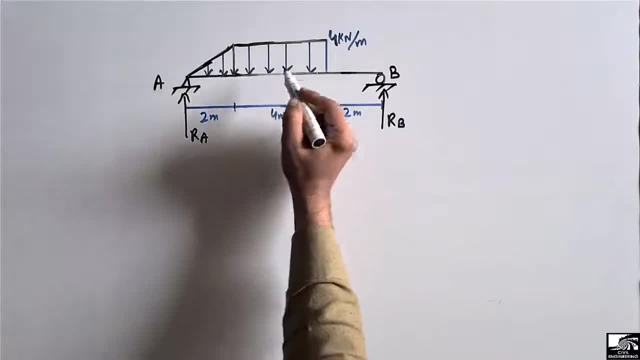 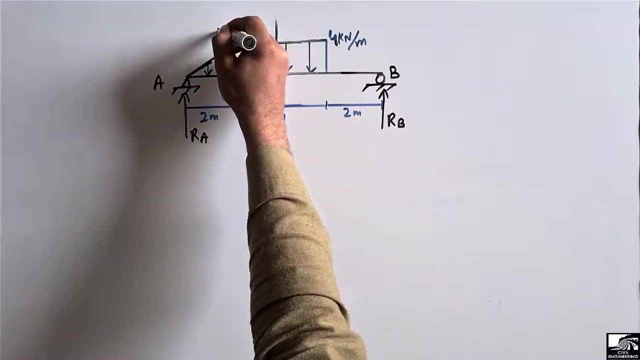 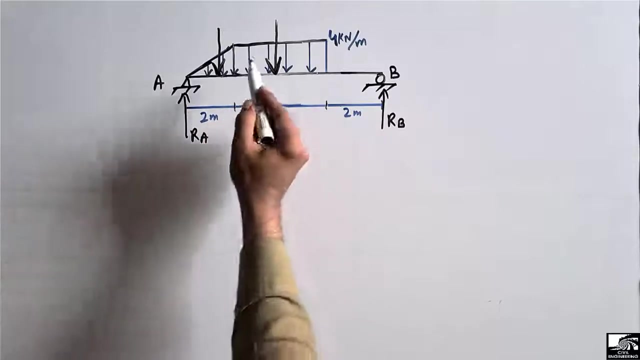 pointed load of each shape. First we have to find out the pointed load of this triangular, of this rectangular, and then we find out the pointed load of this triangle. In order to find out these loads, we have to find out the area of their shapes. 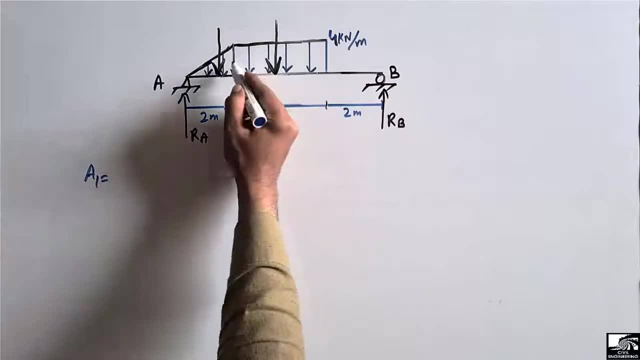 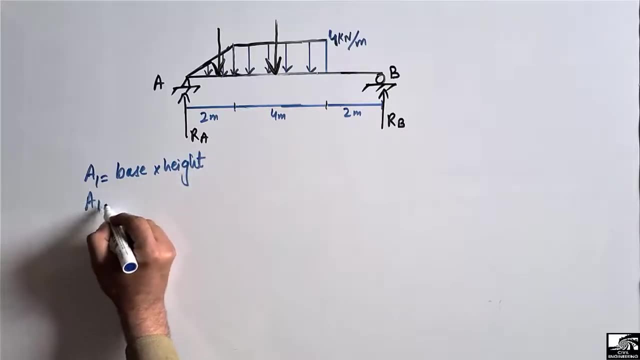 The area. let's consider: the area of this rectangle is based into height, So A1, the area is based into height, So this rectangle has a base of 4 meter and has a height of 4 kilonewton per meter. 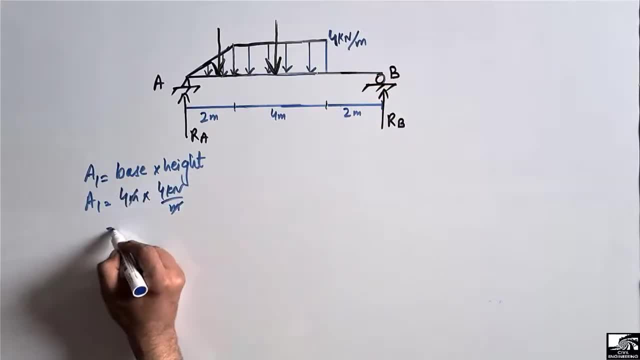 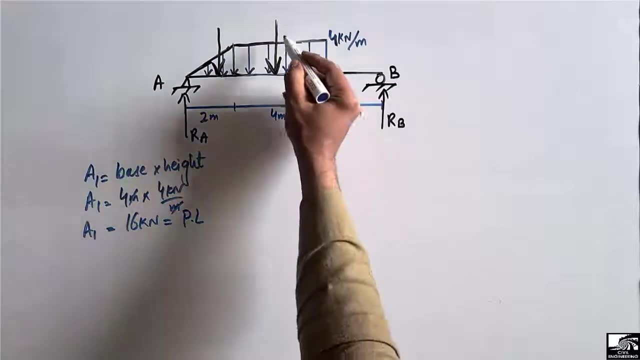 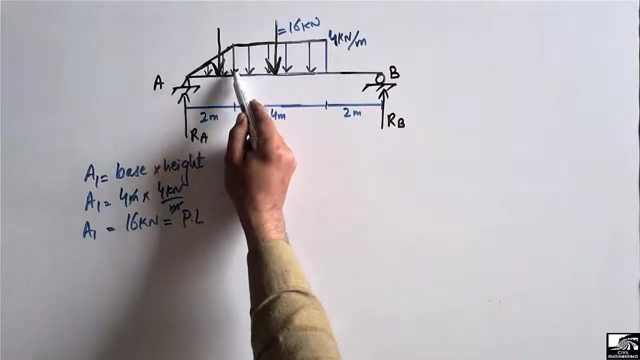 So meter, meter will be canceled. we got 16 kilonewton. So this is the area, or we can say pointed load, of this rectangle: 16 kilonewton. Now, similarly, we will find the area of this triangle and we will find out the pointed load for this triangle. So it is A2, equal to. 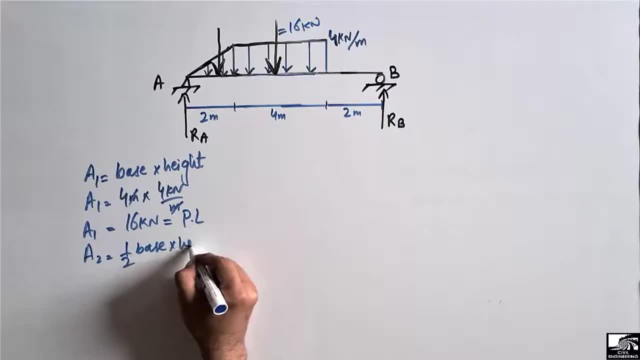 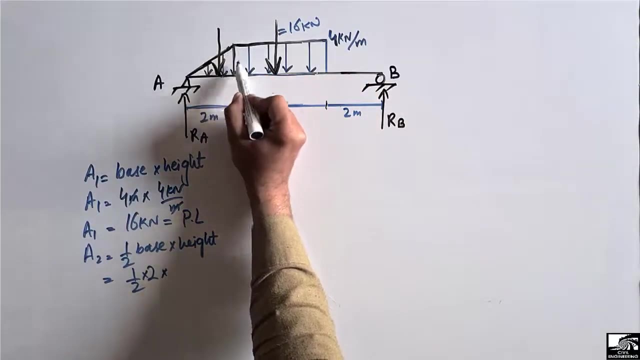 half base into height. This formula is used to find out the area of the triangle. Now, half base is 2 meter for this triangle and height is again this: this is the same height, so it is 4 kilo Newton because this height of the triangle goes. 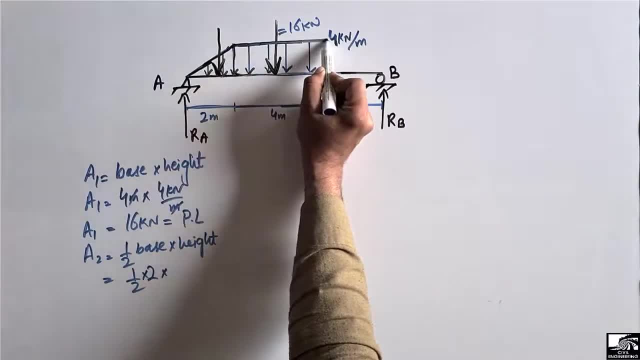 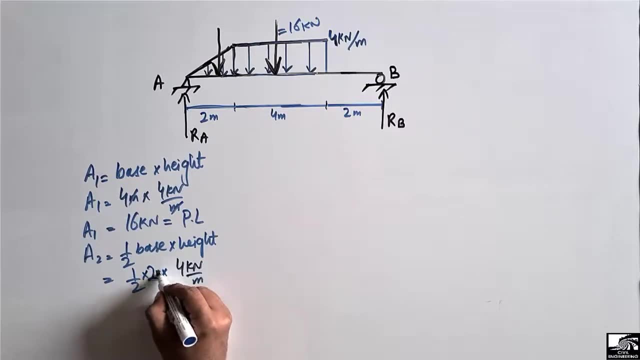 from this point up to the end of the load. so this is also 4 kilo Newton per meter. so height is again 4 kilo Newton per meter and this was 2 meter. so meter will meter will be cancelled and we got 4 kilo Newton. so we have A2 or we can say: 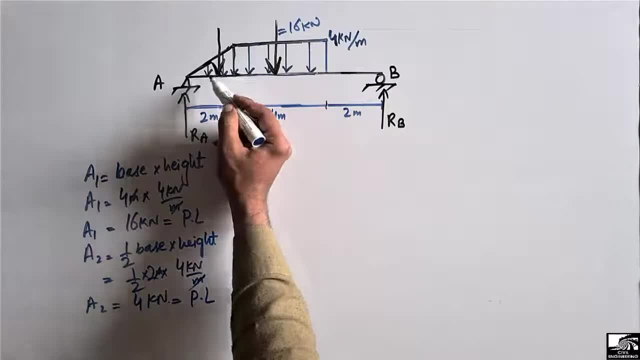 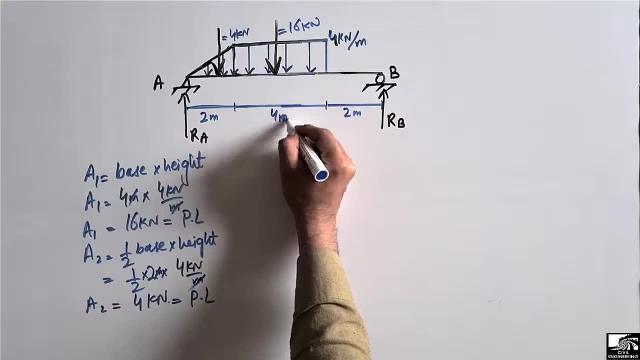 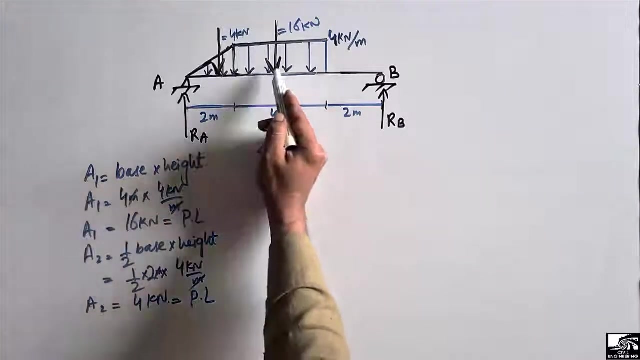 the pointed load acting on this triangle is 4 kilo Newton. so we find out the total load, total pointed load acting on each of the shape of the load. first was the rectangle and then it was the triangle. now it's easy for us to find out the moment. 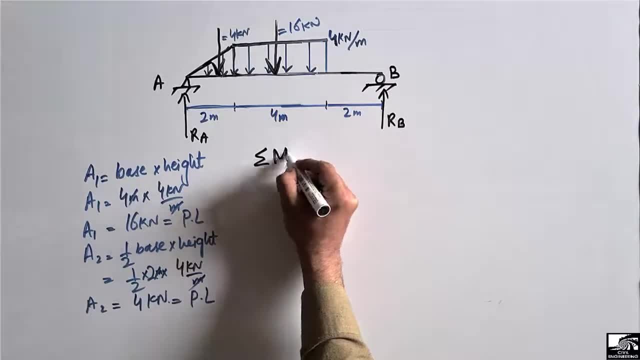 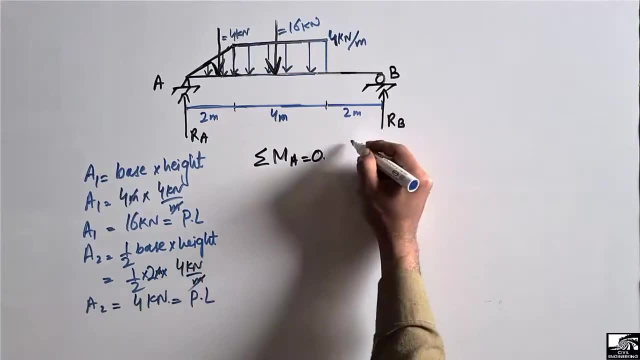 so let's see: consider summation of moment at point A equal to 0. to find out the summation of moment at point A equal to 0, we have to take the clockwise moment is taken as positive in the anti-clockwise moment is taken is negative. this is just our sign. 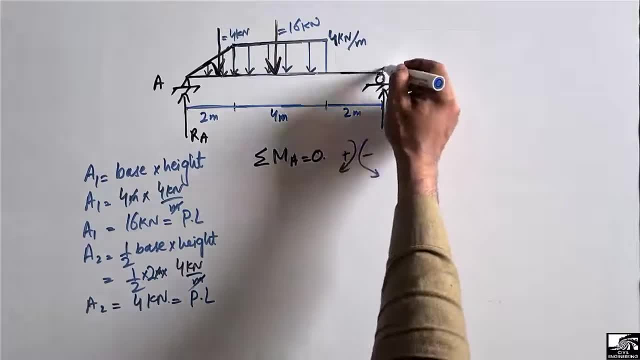 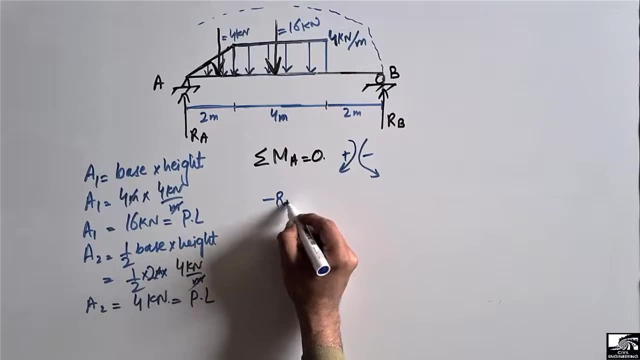 convention. so RB force will create moment in the anti-clockwise direction about point A. so it will be minus RB multiply with the momentum. the momentum is the distance from the point A to the point B, so it will be minus RB multiply with the momentum this particular force will create the distance from this B. 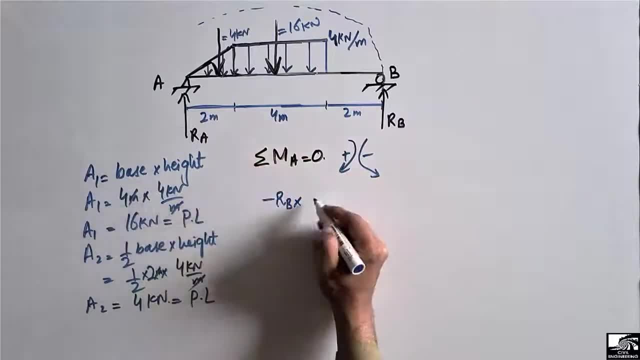 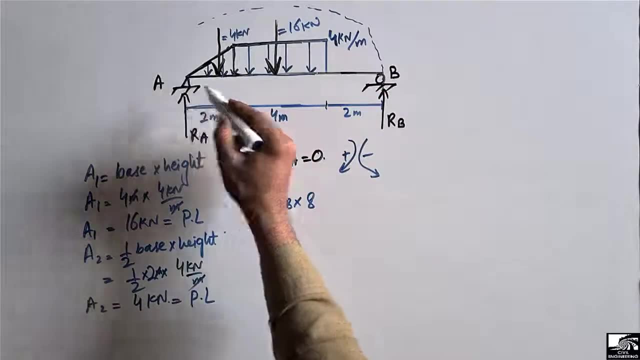 point up to a, which is 2 plus 4 plus 2, which is 8 meters, and then this load is from this B point up to A, which is 2 plus 4 plus 2, which is 8 meters, and then this load also creates a movement rectangular load about point A and it creates a. 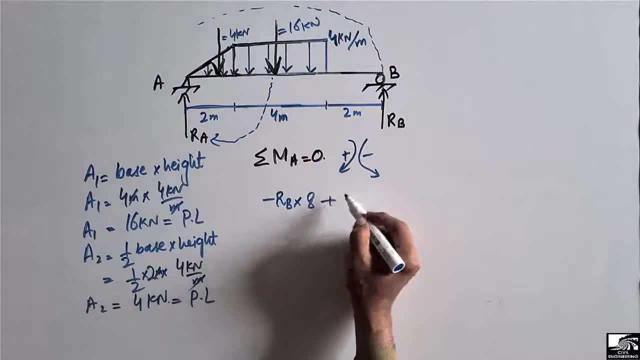 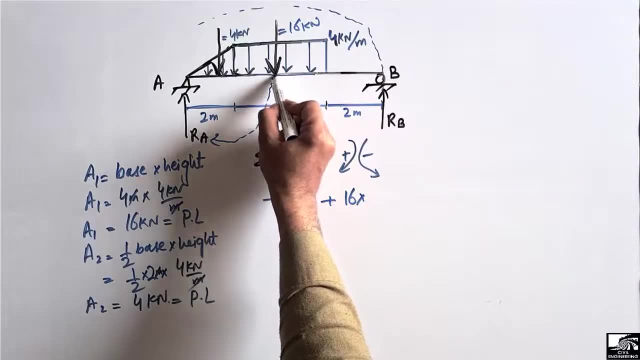 moment in the clockwise direction. so it will be plus 16 multiplied with the moment. all the movement arm is the distance from this centroid rectangle up to point A. so it is half of before, which is true. this road will be half of the. this one is bottom half of the force. so this, that this leg isErg moment based on 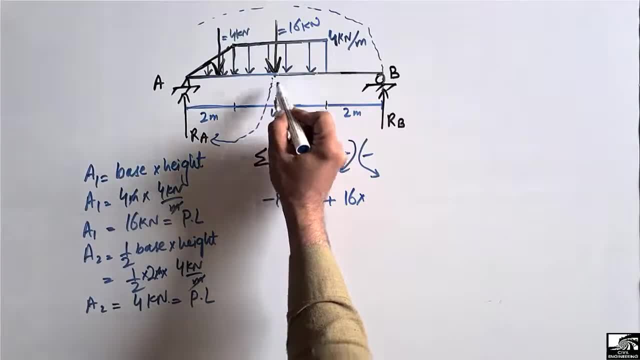 so that we are Edge close by the point above because it is Makes no difference. This we determine that the full upper jealousy it also creates this avant- dramatical. this наших gotta fallen for a bit because it is part of the direction above the blunt based. 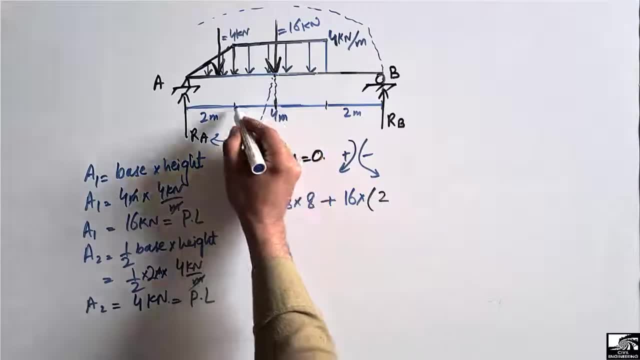 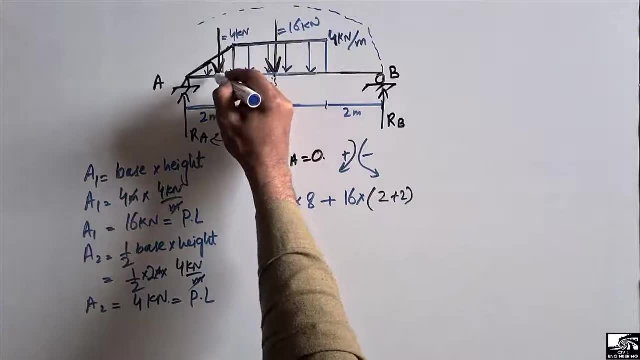 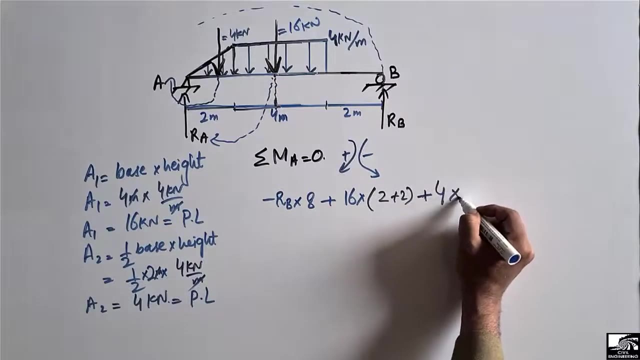 half of the 4, 2. this 2 plus 2, so the total will be 4. then again, this load, triangular load, also creates a moment about point a in the clockwise direction, so it will be again taken as positive. and 4 kilo Newton multiplied with the: 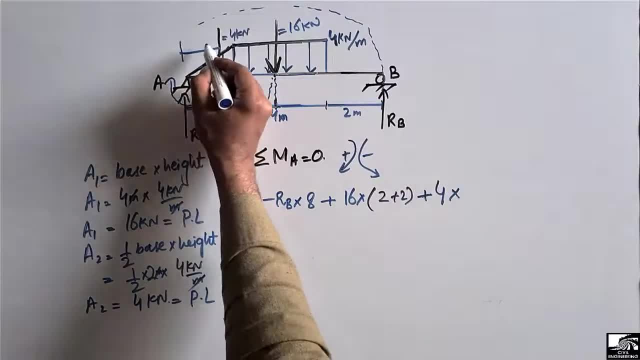 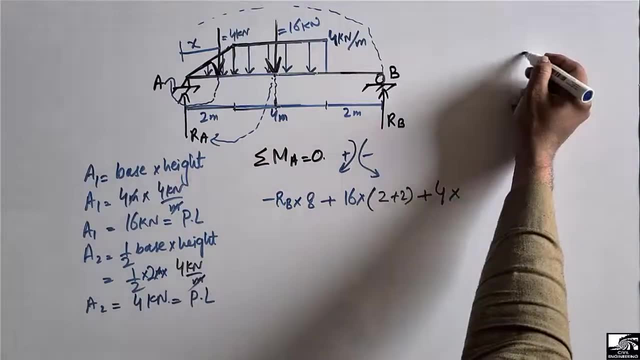 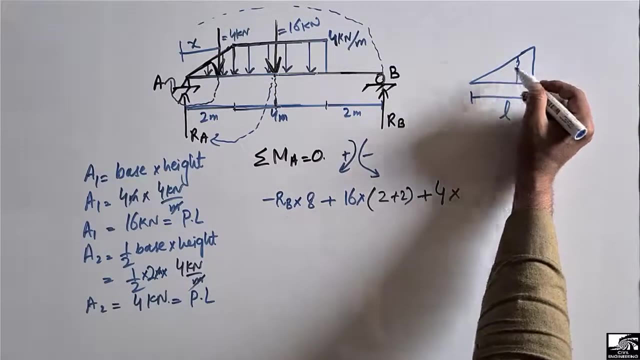 momentum. the momentum is distance from this point up to this 4 kilo Newton, so this is X. this is unknown to us. so if this is in a triangle, let's suppose total length of L, so the centroid lies at 2 third of L from this end and from. 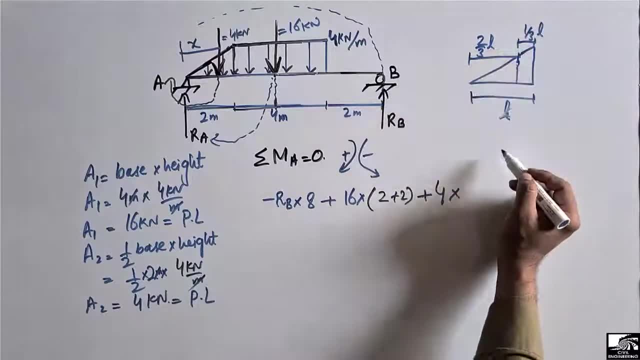 this end up to this point, it will be 1 third of L. so, similarly, from this end up to this point, it will be 2 third of L. so it will be 2 third of L, where L is the length of this triangle, which is 2 meter. 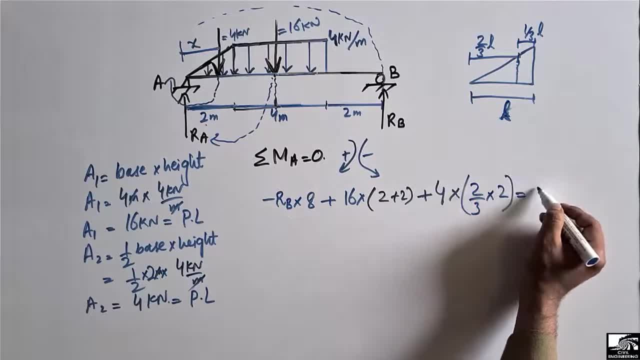 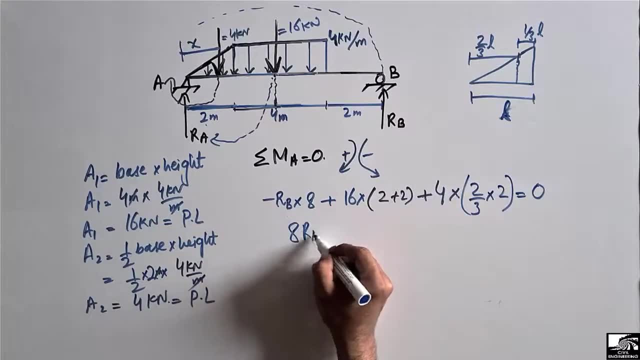 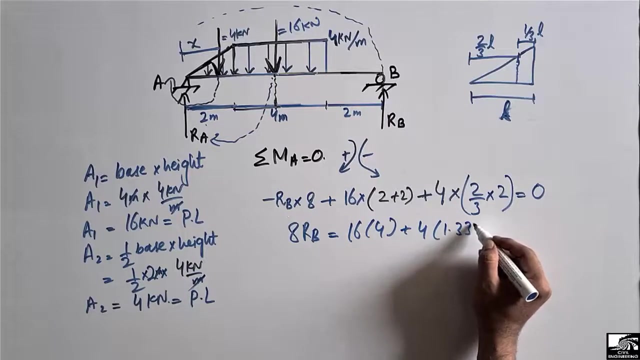 so this is the way how to find out the summation of movement at point a, equal to 0. now it are. B will be shifted into the right side, so we get 8. 8 RB equal to D. if we multiply all these quantities, so we get 16 into 4 plus 4 into 1.33. 8 are B. 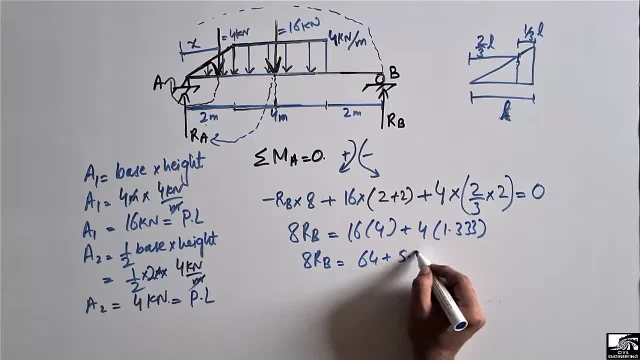 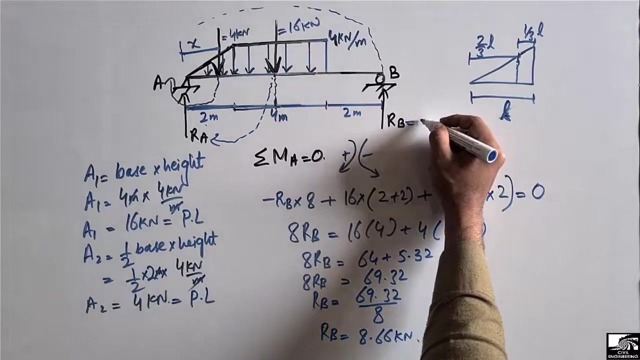 will be equal to the 64 plus 5.32. so we got 69.32, 8 RB and RB comes out to be 69.32 divided by 8. we got RB equal to the 8.66 kilonewton. now this is the support reactions at support B, 8.66 kilonewton. similarly, we will 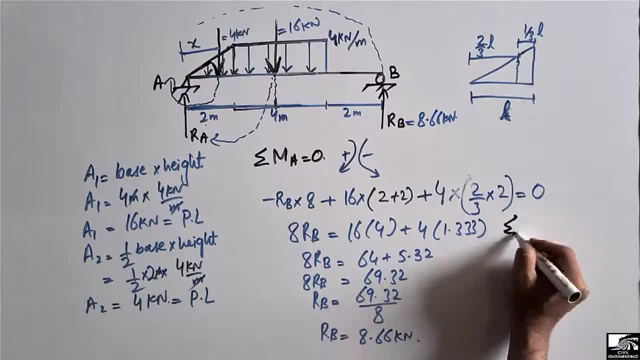 find out, the support reactions are a. so by using this equation, summation of vertical force is equal to 0. the upper force is taken as positive in the downward forces are taken as negative. so the upper forces are R a and R B. so R a and R B are taken as positive and downward forces are 16 kilonewton.